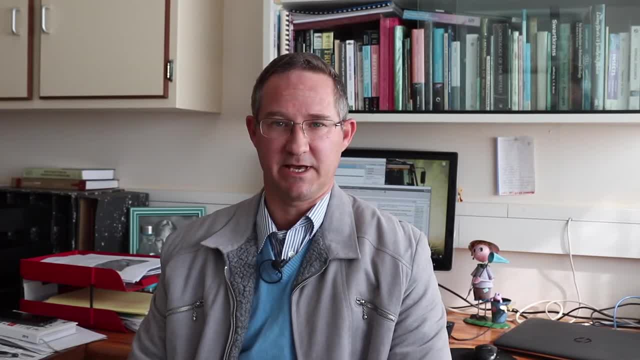 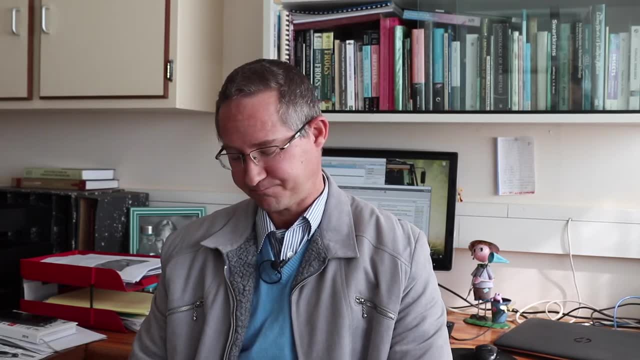 It's also one of the few courses in the module where you will be doing an excursion and getting hands on experience on how to work with the various taxonomic groups. Then we get to the elective modules within the curriculum, The first of which is OMBO 613.. 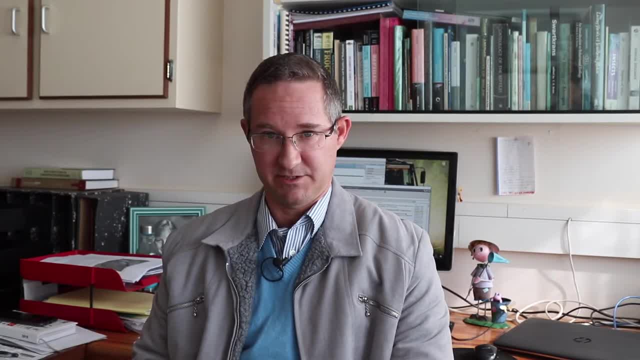 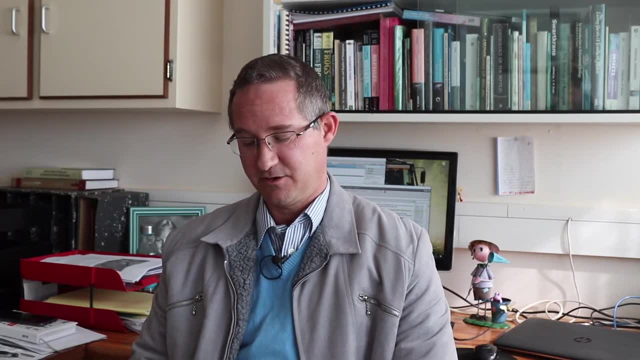 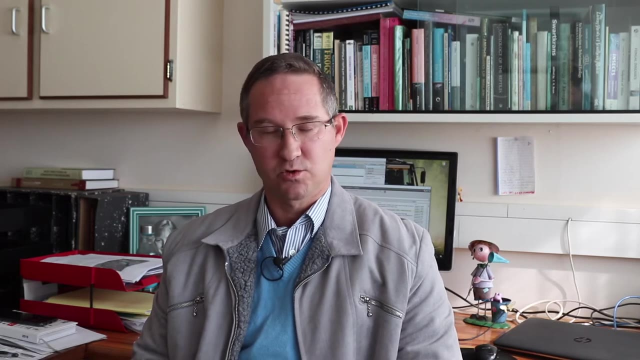 It's Introduction to Environmental Management. This provides a background and a foundation for you into environmental management processes. It looks at the various instruments in which to measure environmental management, how to apply these processes, and it also includes environmental law and legislation in the module. 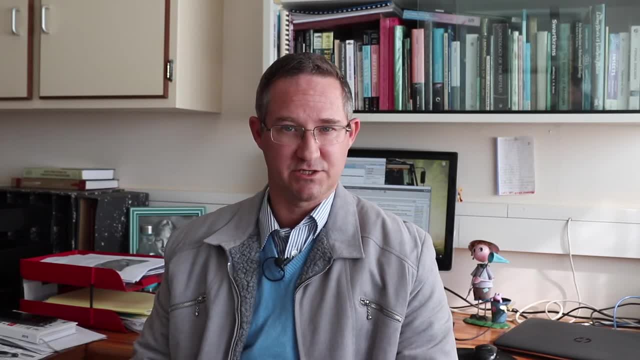 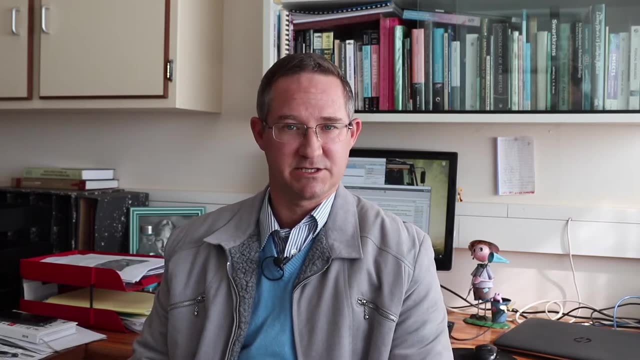 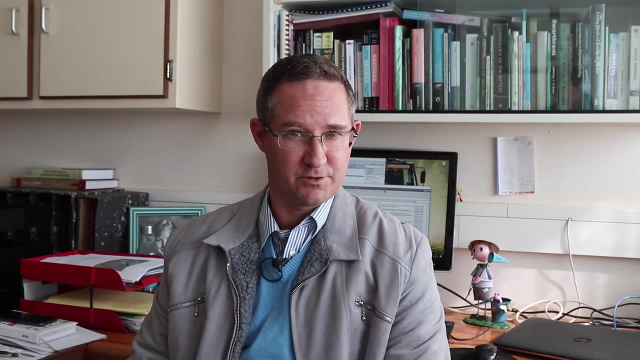 Secondly, we have OMBO 613: Introduction to GIS. For those of you that are interested in drawing up maps using large data sets of environmental data, anthropogenic layers like urban development, etc. This is the module for you. It's got a lot of modern application: internal and regional planning, environmental management. 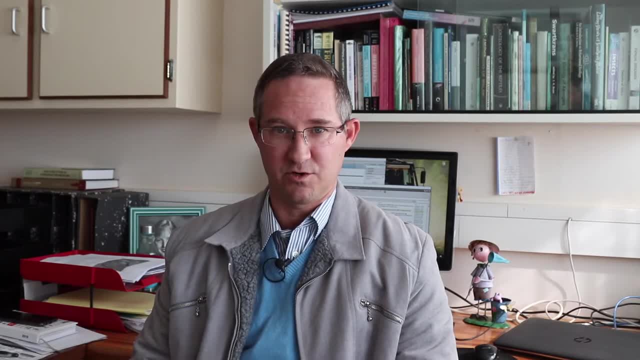 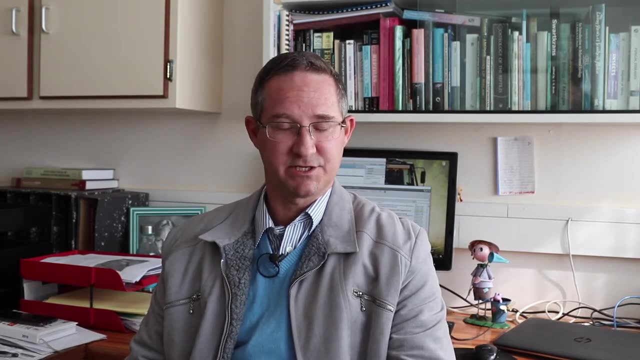 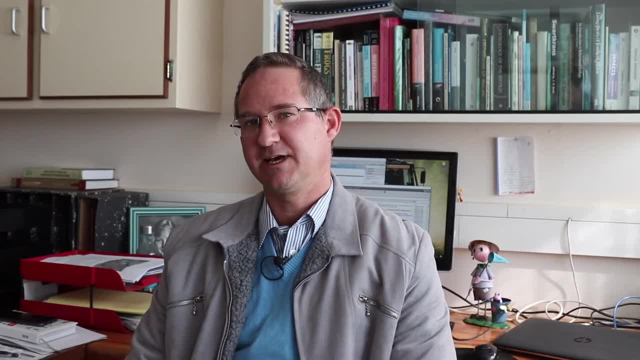 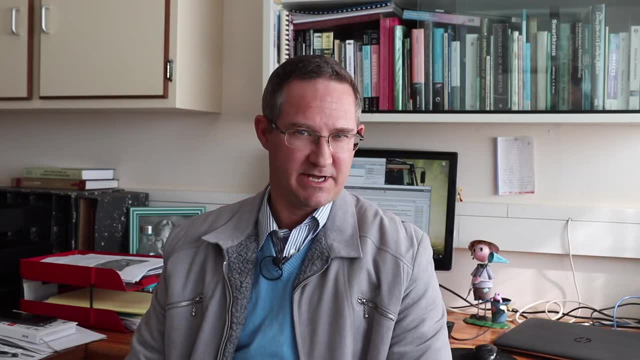 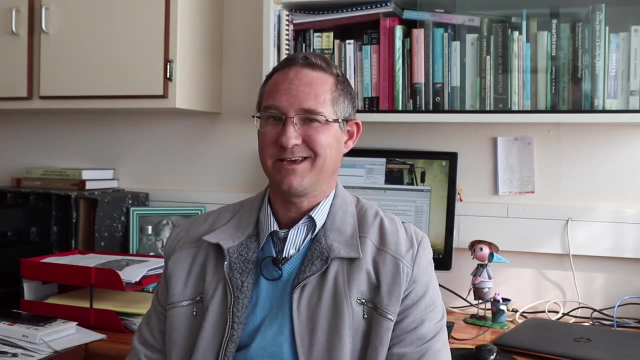 So this module is a taxon specific module. You'll be studying the biology, the ecology, the behaviour of amphibians and reptiles and in practice. So that is how to become a herpetologist: Either in an academic environment, like research at universities, or either in the industry. 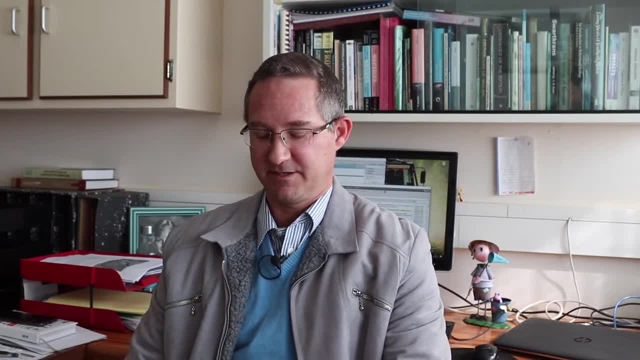 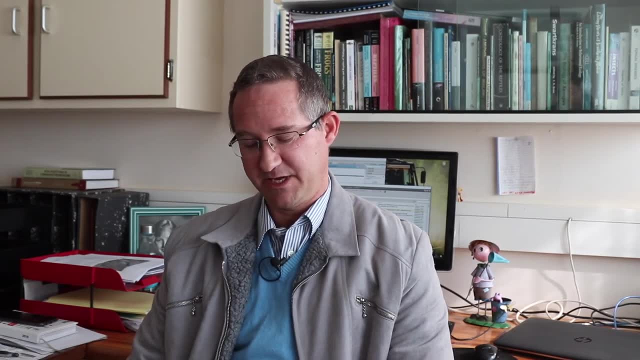 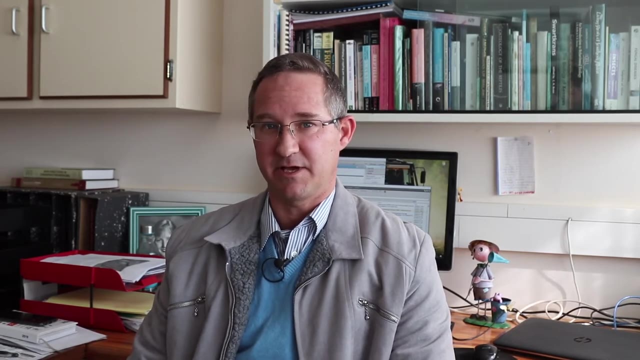 when you want to do environmental management, biodiversity surveys. This is a really good course to take if you're interested in herpetofauna in South Africa. OMSB 628 is coral reef ecology. So again in this module, it's very specific and focuses on the habitat of ecological or 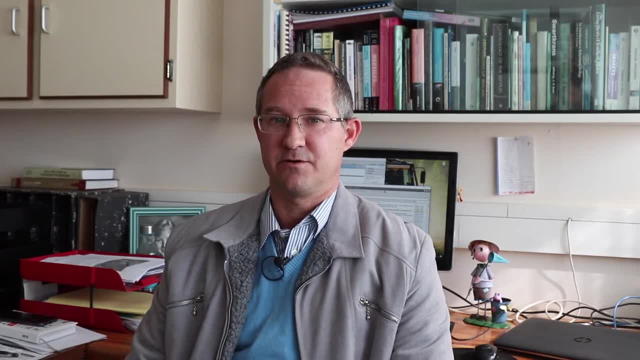 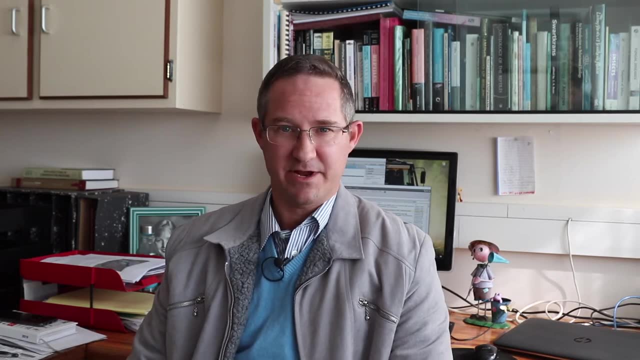 of coral reef ecosystems. So, as you might know, this is a very, very sensitive habitat. It's under tremendous threat, So any threats to the marine environment directly impacts the coral reef ecosystem and it's very rich in biodiversity Of both invertebrates and vertebrates, such as fishes and sharks. 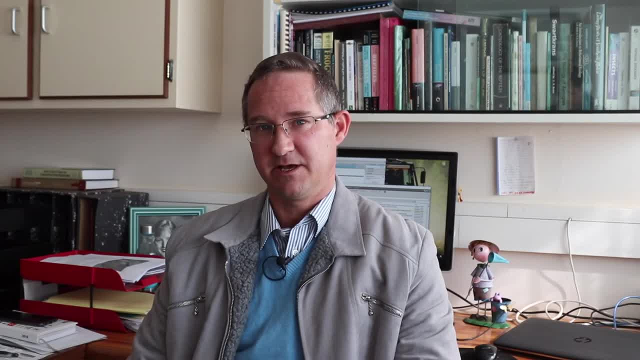 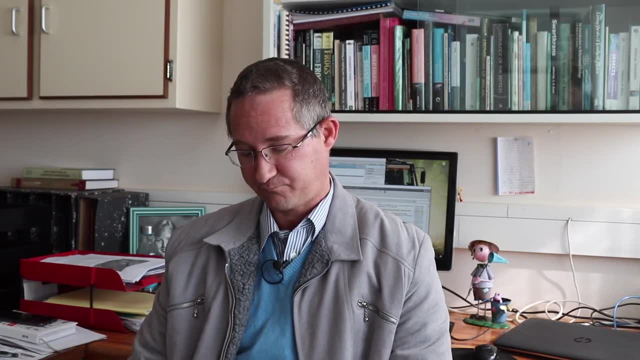 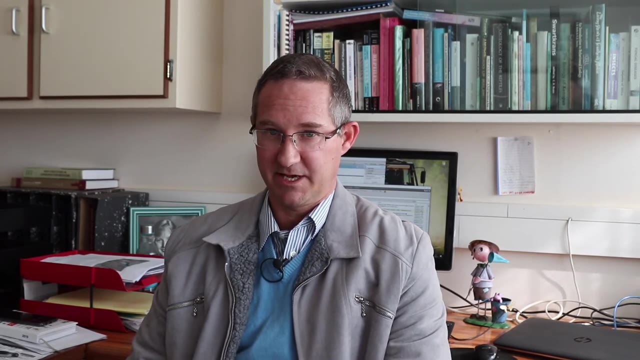 And in this module you learn about that sensitive interplay between ecological management systems, as well as the threats and the conservation implications thereof. OMSB 629 is genome analysis and bioinformatics. In modern biology and environmental sciences you can't go wrong without looking at bioinformatics. 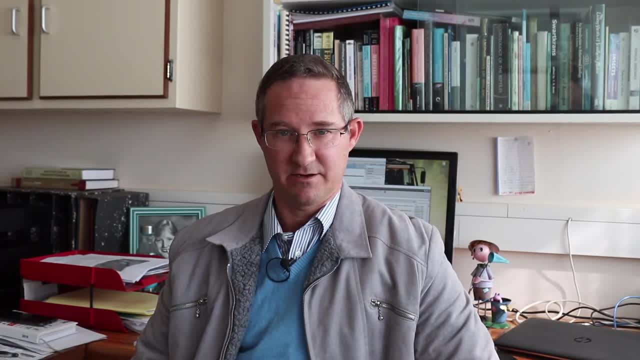 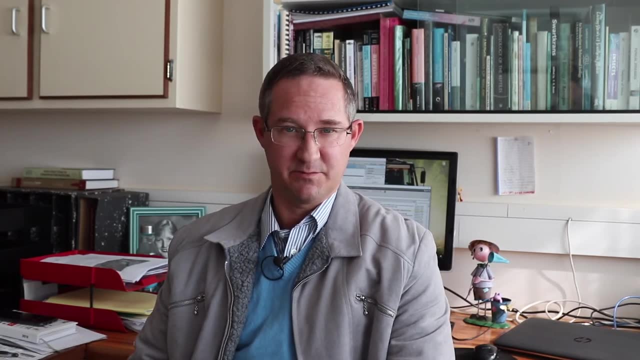 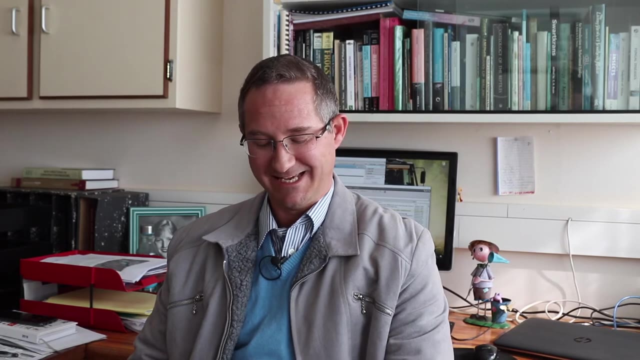 Genomic analysis and molecular analysis, And that's exactly what you will be doing in this course, So you will be exposed to various molecular systematic tools and learn how to interpret systematic data as well. OMSB 621 is restoration of degraded ecosystems. 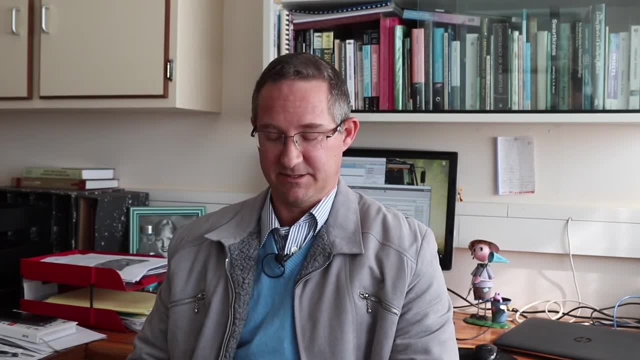 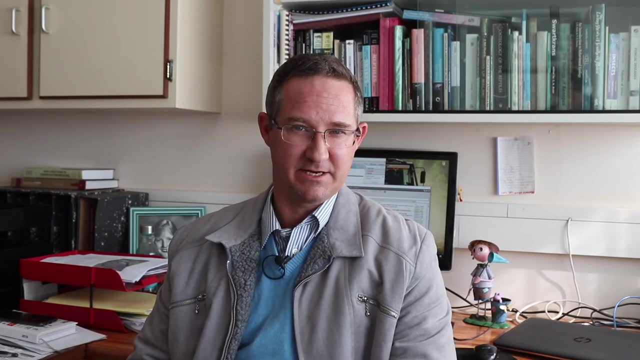 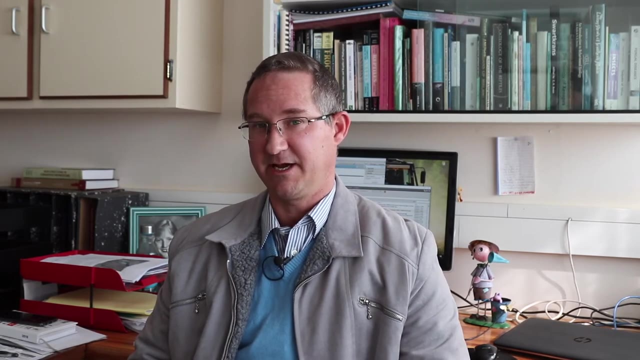 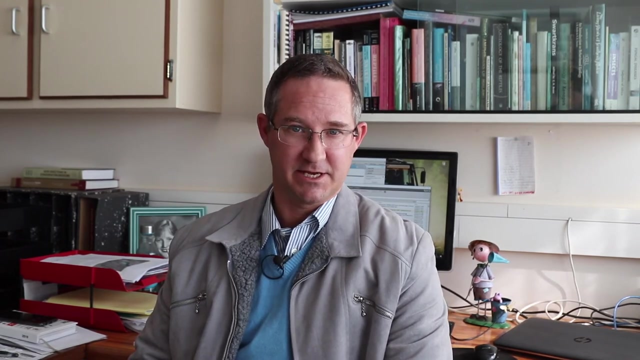 So this module focuses specifically on the terrestrial ecosystems And the threats thereof, And how to manage land and environmental systems in the terrestrial environment. So students will learn about sampling and gathering data in terrestrial ecosystems, as well as how to apply multivariate statistical analysis in interpreting those data. 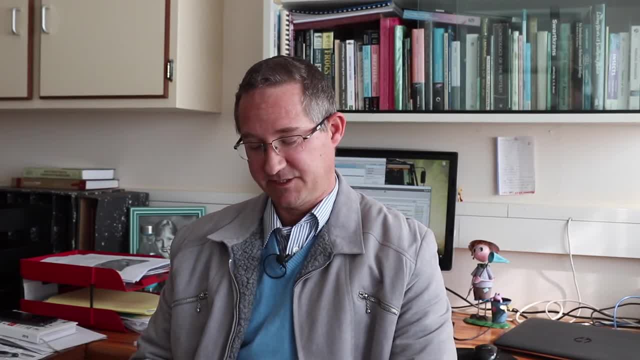 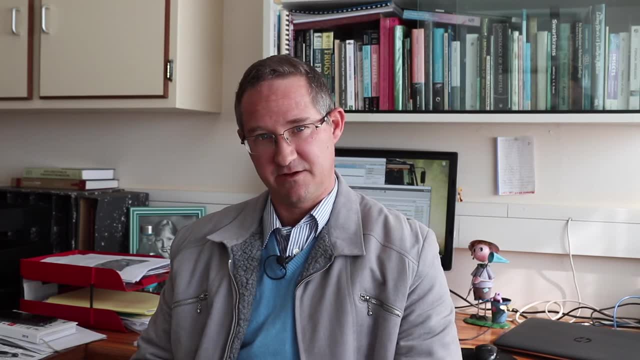 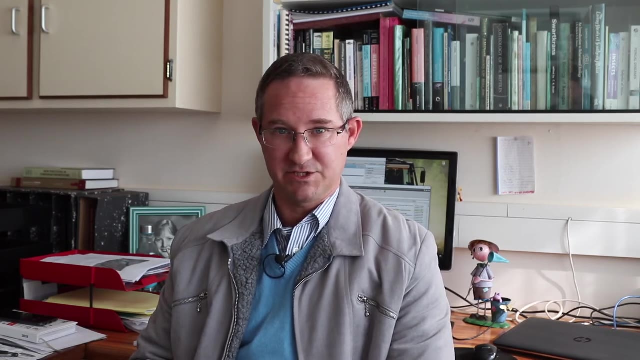 OMSE 625 is advanced ecotoxicology. It's the study of threats in the environment on biodiversity. So these can be chemical threats. They specifically have to do with anthropogenic involvement. So what's the role of humans and industry, and perhaps even agriculture, on the functioning 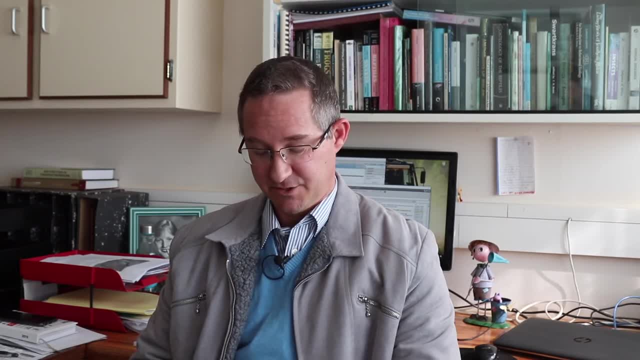 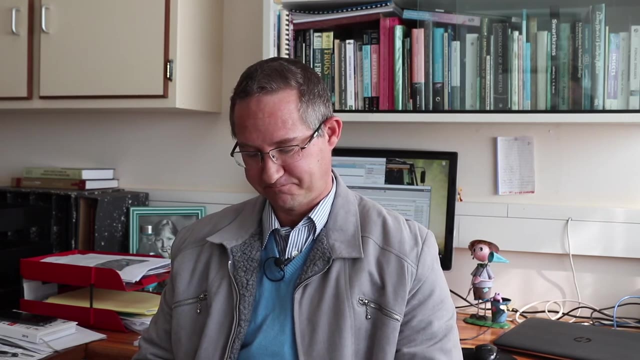 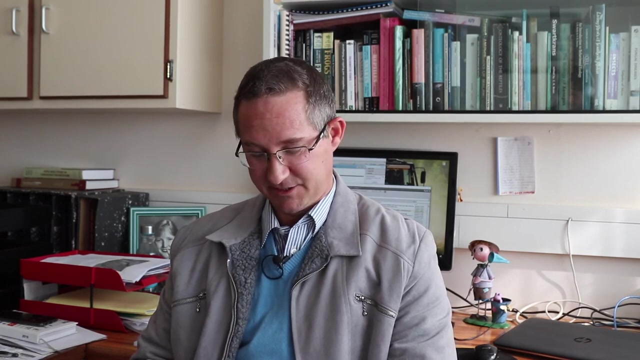 of ecosystems and biodiversity specifically. So again, you will be looking at methods on how to sample biodiversity and search for specific toxicants within those biological tissues, And again, how to interpret those data. Finally, the last elective module that you might opt to choose is OMSP 624.. 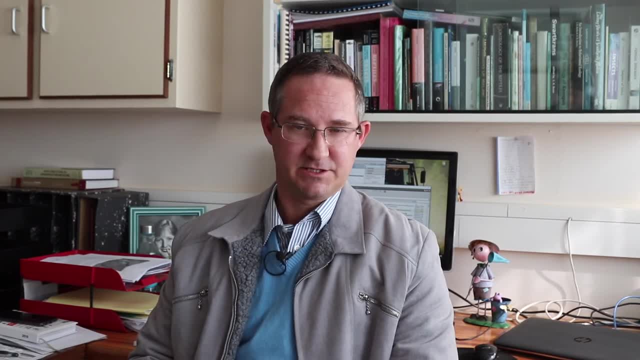 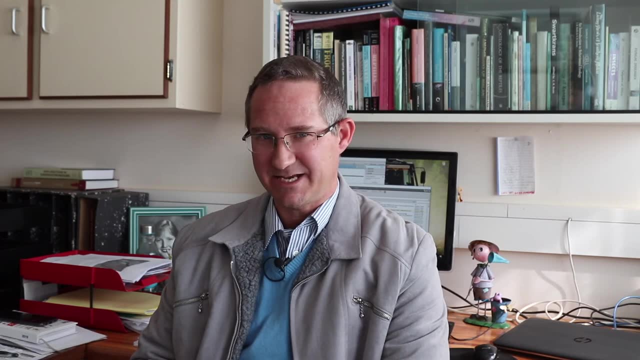 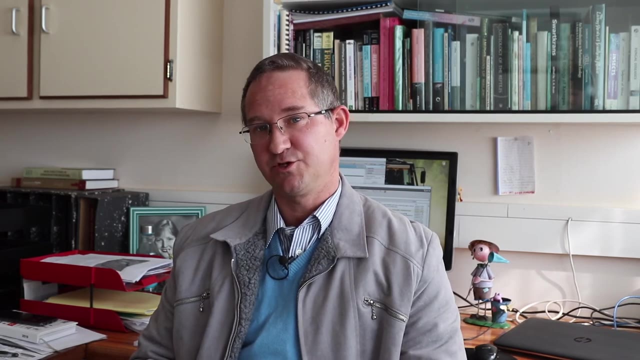 And this is the arthropoda plant interactions. So this is a fusion between biodiversity studies and agricultural studies And specifically, the role that insects play In The agricultural systems, and these are insect pests. so you'll be looking at ways in which to monitor the effect of insect pests in the agricultural environment and how to develop.